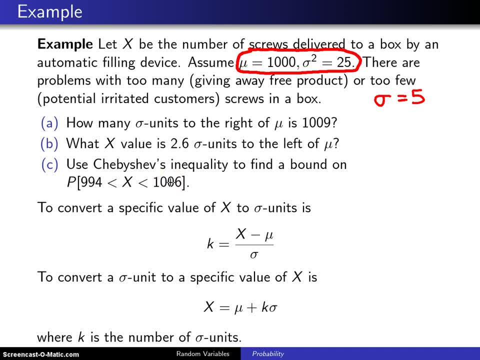 Now, in this particular example, you do not know the exact shape of the probability distribution. You don't know if it's bell-shaped or if it's skewed a little bit to one side or the other. There's no information given other than the population mean and the population variance, So we can't lean on a distribution such as the normal distribution. to answer this, 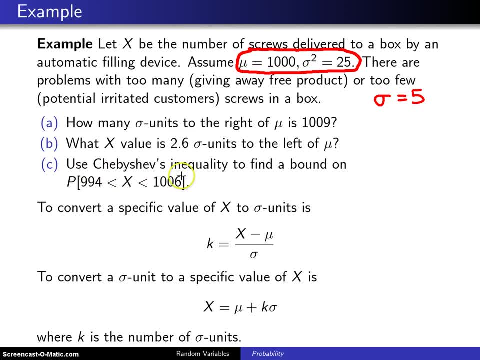 We can only get a bound on this particular probability Using Chebyshev's inequality. before we start out on prop parts A and B to the problem, here are a couple of formulas to convert a specific value of x to sigma units. You can use the formula: k is equal to x minus mu divided by sigma. 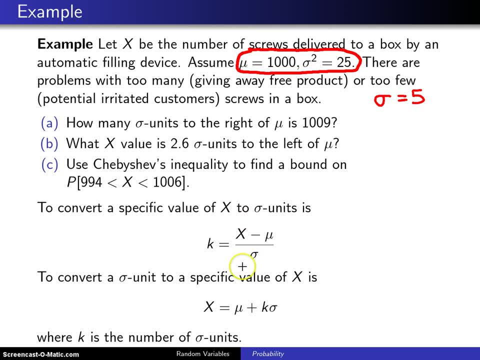 This might look familiar from earlier in the chapter and that is the standardizing where you subtract the population mean and divide by the standard deviation. If you subtract the population mean and divide by the standard deviation. If you subtract the population mean and divide by the standard deviation. 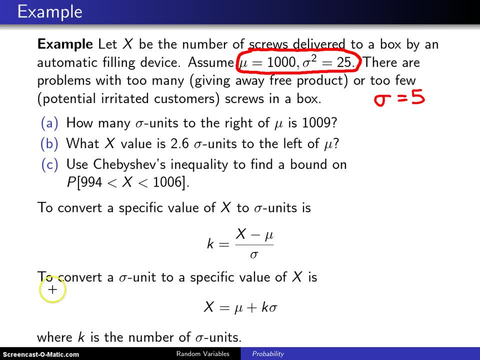 If you solve this equation for x, you can convert a sigma unit- and that's what we're doing in part B- to a specific value of x, by saying x is equal to mu plus k sigma, where k is the number of sigma units. 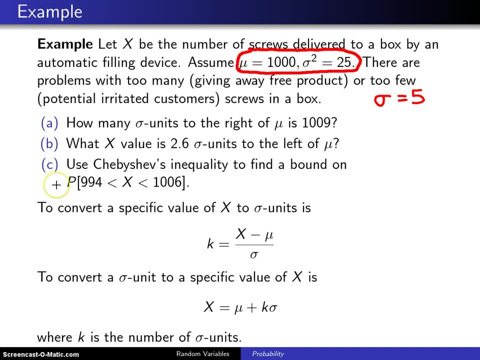 So at this point we're going to answer parts A, B and C. The first part is how many sigma units to the right of mu is 1009.. The second part is how many sigma units to the left of mu is 1009.. 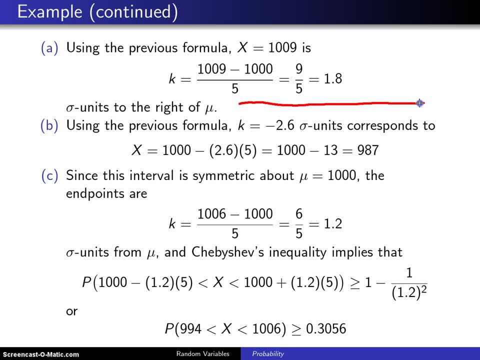 Let's go ahead and draw a picture here. We know that the center of the distribution is at 1000. And we know, because the standard deviation is 5, we can go ahead and draw points along this axis that correspond to sigma units. 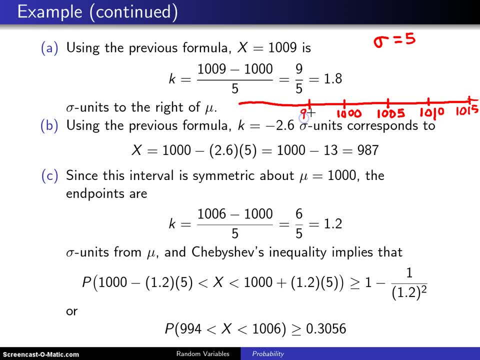 there they are going to the right and you can do those same in units of five off to the left. So when the question is how many Sigma units to the right of mu is a thousand and nine, you can see over here: a thousand and nine appears right. 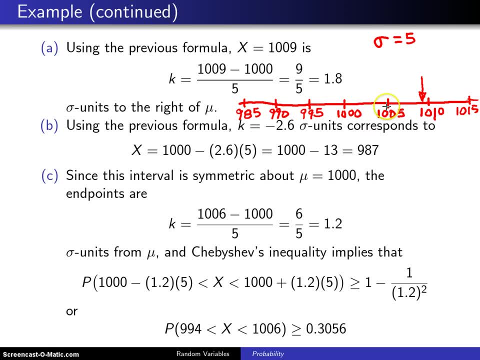 here, and if each tick mark here is a Sigma unit, then it is one point eight Sigma units to the right, and that is calculated by taking a thousand and nine minus a thousand divided by the standard deviation five, and that is nine fifths, or one point eight. 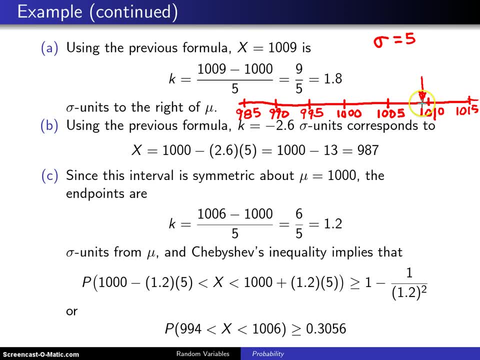 So you can measure this in absolute numbers associated with the random variable, and this would be nine screws to the right of a thousand. or you can measure it in Sigma units and in Sigma units. this is one point. eight Sigma units to the right of mu. Now the question going in the other direction. 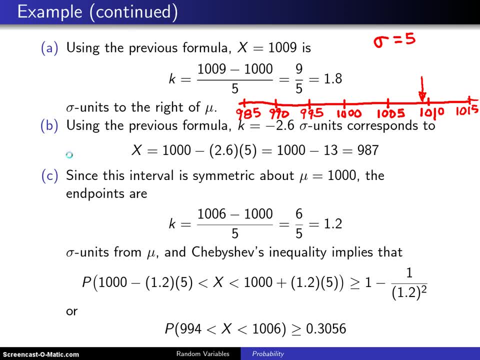 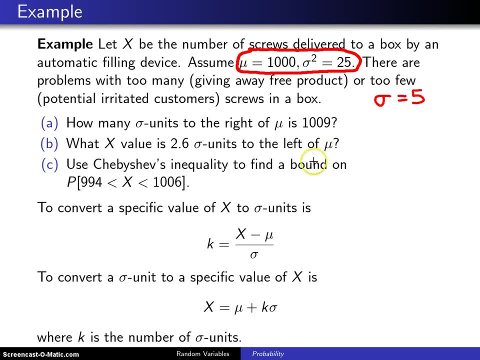 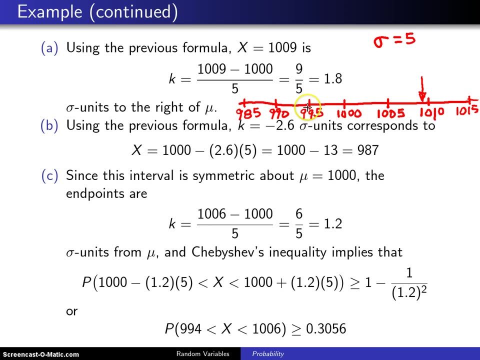 and this is part B. the question in part B was what X value is. two point six Sigma units to the left of mu. if you go to our number line and started a thousand, here is one standard deviation of the left, two standard deviations to the left and two point six standard deviations is about right here. 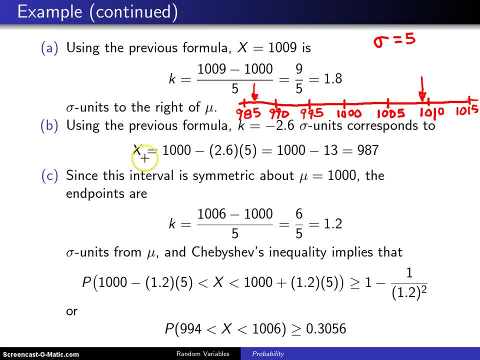 so how is that calculated? we use the second formula this time. X is equal to mu, which is a thousand, and then we put in our K value here, which is one point eight gamma units to the left of mu. so that gives you one point eight Sigma units to the left of mu. 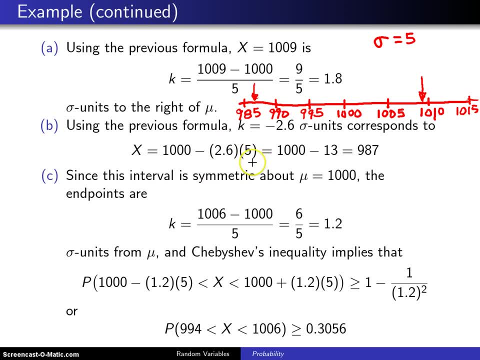 which is negative, 2.6 times the standard deviation, which is 5.. 2.6 times 5 is 13.. 1,000 minus 13 is 987.. So parts A and B show that we can convert from specific values of x to sigma units. 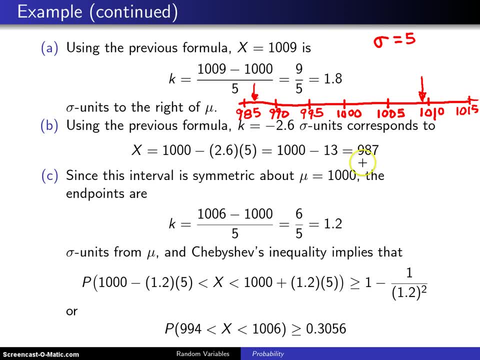 and from sigma units to specific values of x. Finally, part C is to use Chebyshev's inequality to get a bound on the probability that there are between 994 and 1,006 screws in the box, And that happens to be a symmetric interval about 1,000,. 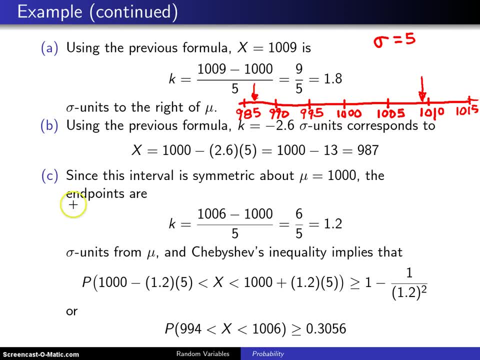 which means Chebyshev's inequality can be used, And the endpoints of that inequality are: K is equal to 1,000, 1,006 minus 1,000 divided by 5,, 6 fifths or 1.2 sigma units from mu.